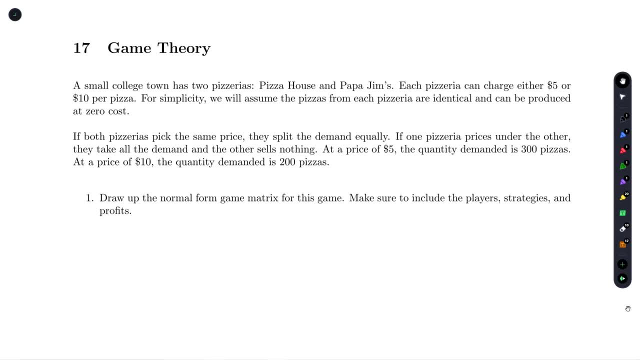 Hello everyone, I'm Sebastian Y and this is Principles of Microeconomics. In this video I'm going to solve this exercise on game theory. As always, I highly recommend you attempt the exercise first and then watch the video. Here we have a simple price setting game where we have two firms who are competing with each other. They can charge either $5 or $10. We're going to assume that if they both pick the same price, they split the demand equally, and if one price is under the other, they take the entire market. 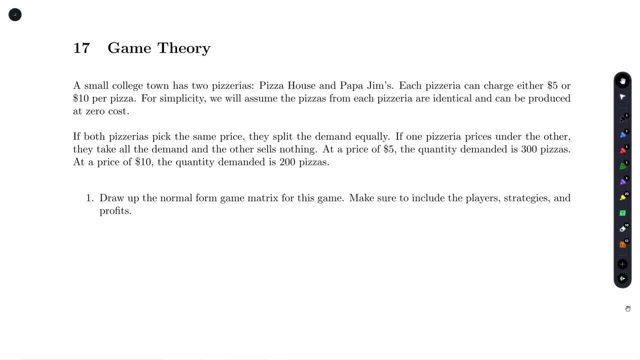 We're given a little information about the demand function. that tells us, at a price of $5, we have a quantity demanded of $300, and at a price of $10, a quantity demanded of $200.. We can use this information to draw up our game matrix. 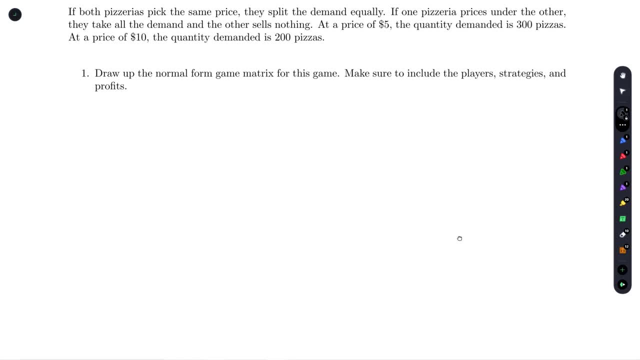 Since we have two players and two strategies, we're going to have our classic 2x2 game, matrix. So I'm going to draw a box and then divide it up into four quadrants. Our two players are pizza- We're going to have our pizza house- and Papa Jim's. It doesn't matter which one you put on the columns and the rows, just as long as you are consistent about it as you go through. 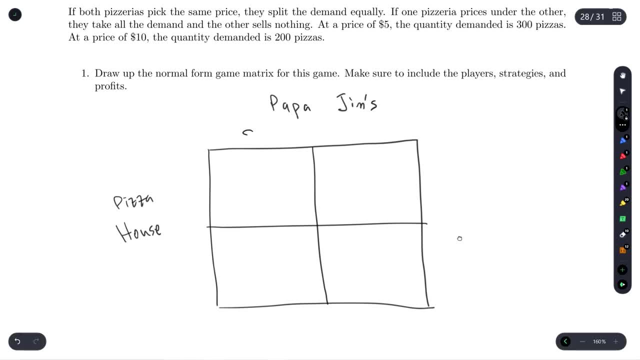 We have two possible strategies here. They can price at $5 and they can price at $10. Those options are the same for each player. Next, we need to think about the profit that they're going to make. The problem stated that we're going to assume, for simplicity, that there are. 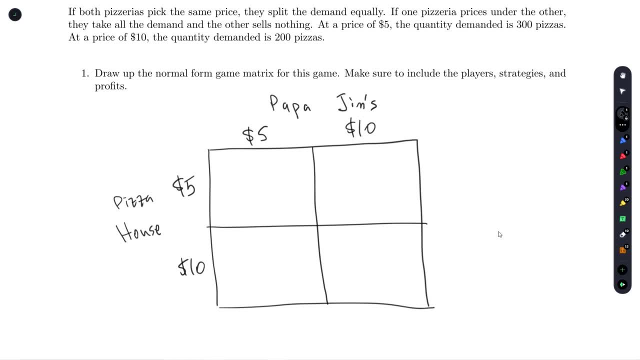 There are zero costs. so we're just going to calculate the revenue for everyone. If both price at $5, they're going to split the total quantity demanded of $300.5, so that's $150 each. So if we're at $5 and $5, the profits are going to be $5 times $150 for each of them, and that's $750.. 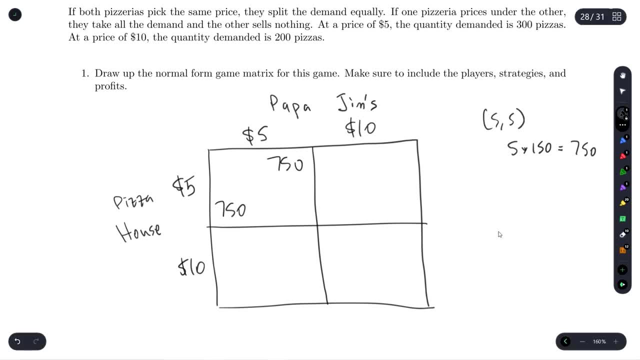 So pizza house is going to get $750.. Papa Jim is going to get $750 as well. I always write the payoffs lower left for the player on the rows, upper right for the player on the columns. Next, if they are both pricing at $10, then they're going to split the quantity demanded of $200.5, and so that's going to be 10 times 100, which is $1,000.. 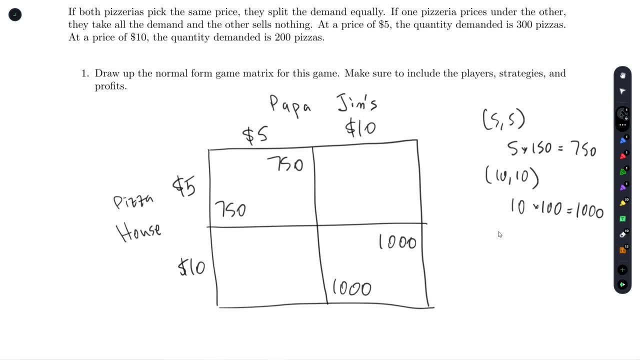 I'll write those in as well. Now we need to see what happens when one of the pizzerias undercuts the other. So $5 and $10 or $10 and $5. In this case, the player who chose $10 is going to sell nothing. So in the upper right, that's Papa Jim's. 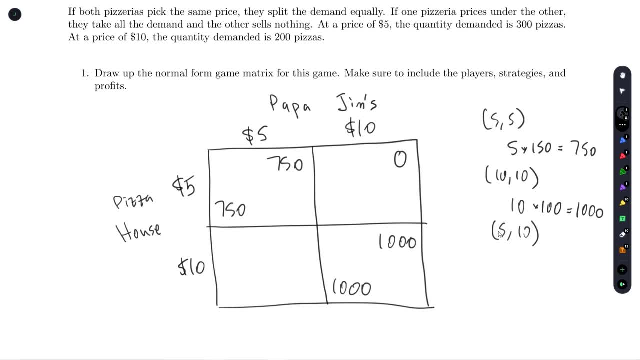 They're going to get nothing and pizza house is going to get the entire demand of $300. So that's going to be 5 times $300, which is $1,500.. If we look at the lower left- this time Papa Jim's is doing the undercutting- They're going to get $1,500.. Pizza house gets nothing. 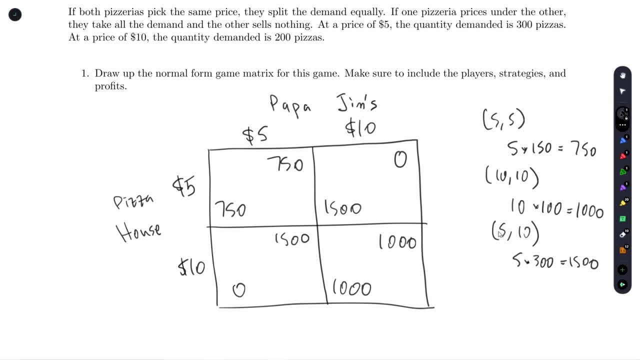 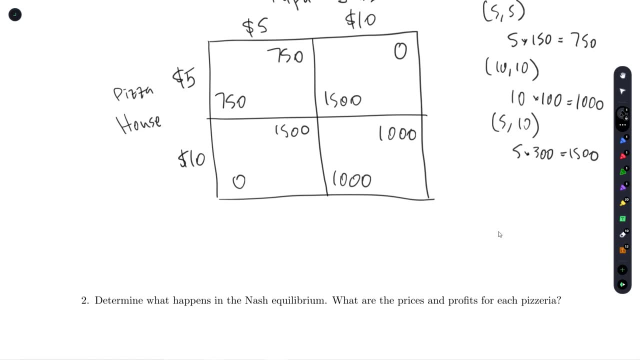 That's our game matrix. Remember that we need to have our three components of a game: players, strategies and payoffs. Next we're going to figure out The way this game is set up. we have a classic Prisoner's Dilemma situation. 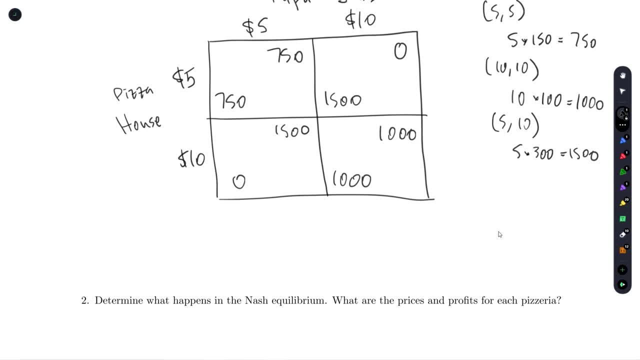 Notice that for pizza house, picking $5 is always better, no matter what. If Papa Jim's picks $5, then pizza house is better off picking $5, because $7.50 is better than $0.. Head: Papa Jim's picked $10.. Pizza house also prefers $5, because $1,500 is better than $1,000. 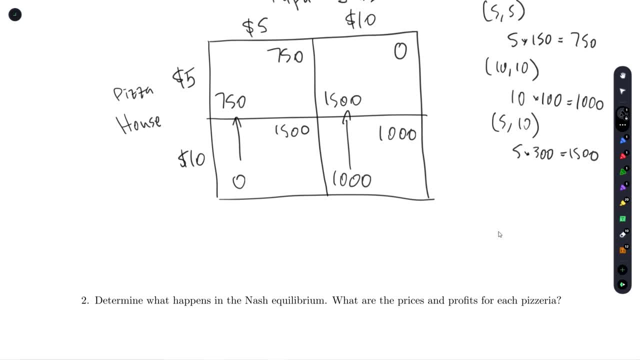 And so pizza house is always going to pick $5, and, since the game is symmetric, Papa Jim's is also going to pick $5. So our Nash Equilibrium is both firms picking $5, and each firm is going to make a profit of $7.50 each. 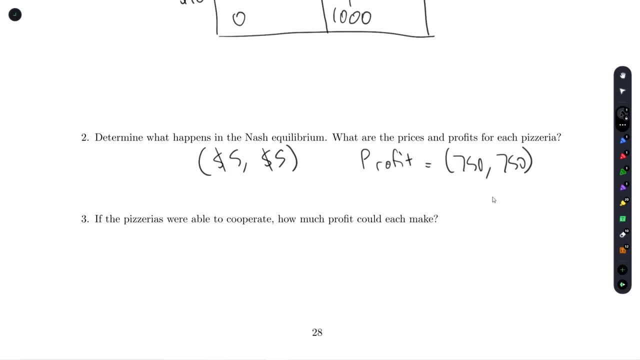 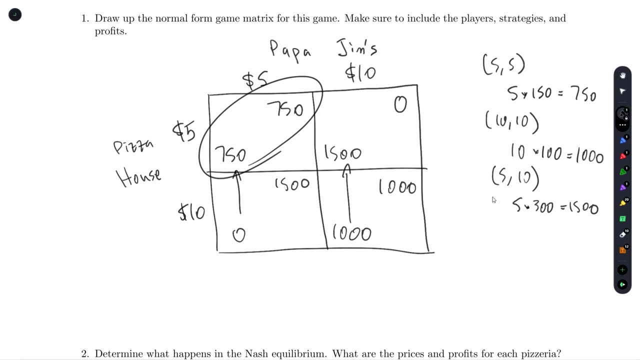 The final question asks us: if they were able to cooperate, how much profit could they make? We can go back up to the game matrix and see In our Nash Equilibrium we're going to end up at $7.50 and $7.50 profit. 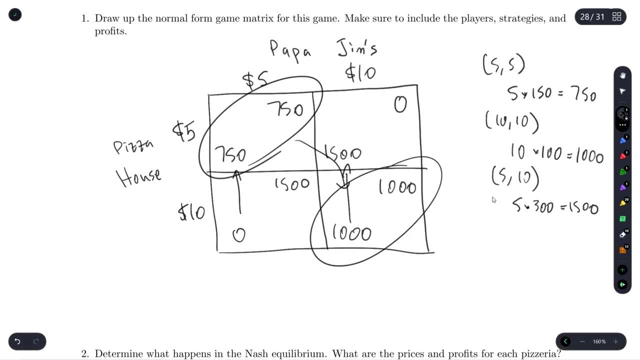 But There is a situation over here where both firms are making more profit- $1,000 each had they been able to cooperate- and both agree to price at $10. Of course that doesn't hold up in the Nash Equilibrium because the self-interested strategy is always going to lead them to pricing at $5.. 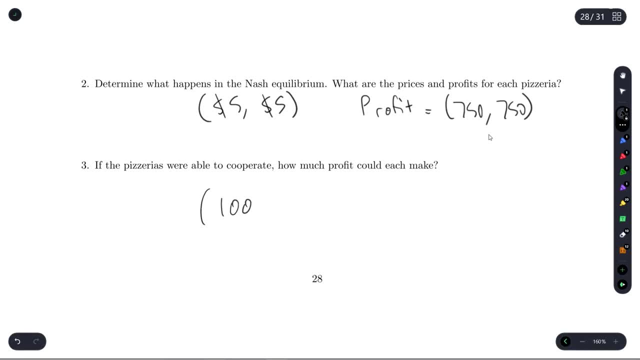 But had they been able to cooperate, they could have made $1,000 each. That's all there is to it. If you have any questions, feel free to let me know. Thanks for watching.